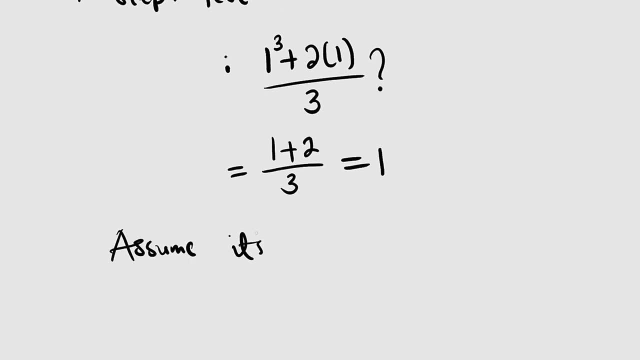 this. the next step is to assume other certain numbers will satisfy. So we assume where k also belongs to the set of natural numbers. So we are going to substitute n equal to k. So we are assuming that k to the third power plus 2k is also divisible by 3.. Let this be true, If it is true, remember. 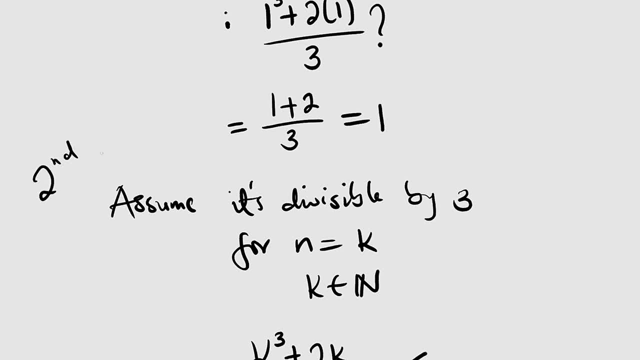 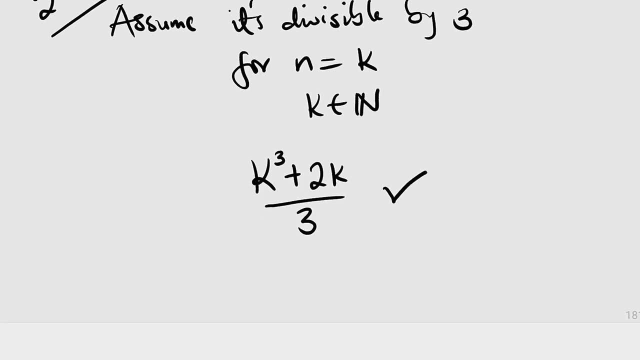 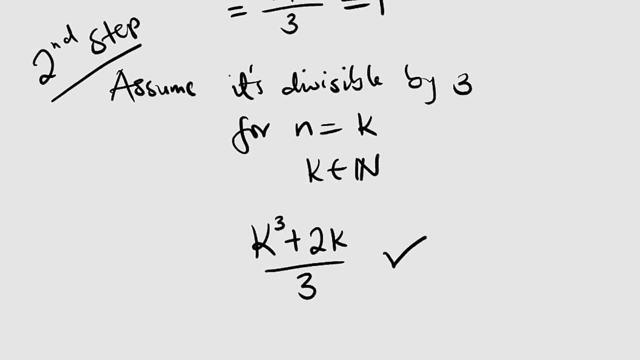 this is the second step. Let me write it here. Second step: This is the second step. We test for k equal to n. So what is the third step? The third step is to replace k with k plus 1.. What does that mean? 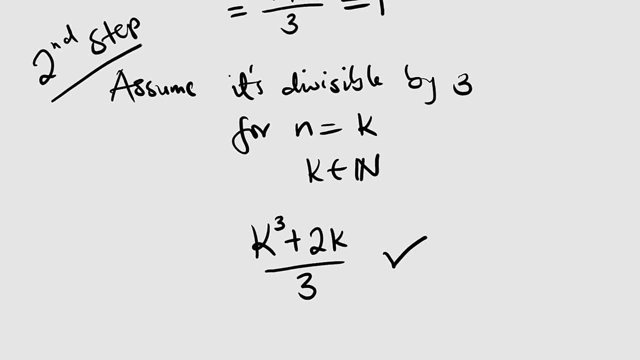 If k is a certain number, for instance 2, if 2 is satisfied, we assume 3 is also satisfied And that will be 2 plus 1, meaning k plus 1.. So let's assume that also k plus 1 will also satisfy this problem. 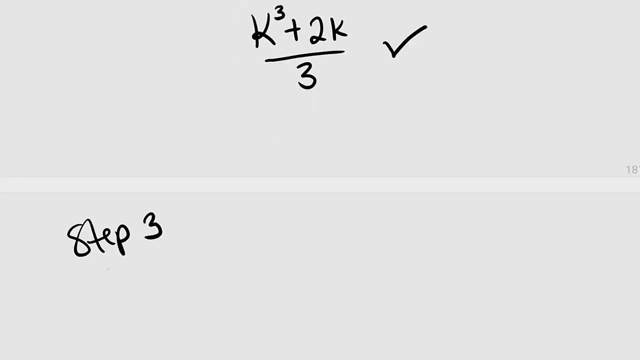 So step 3.. We want to prove that k is also true for some k plus 1.. So we want to prove it is also true for some k plus 1.. So instead of k we replace k with k plus 1.. 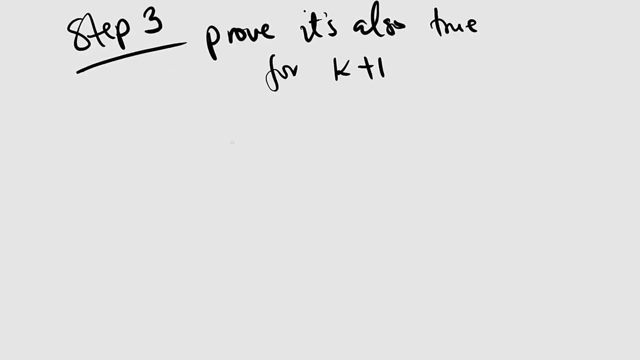 So we want to show that k plus 1 to the third power, replacing k with k plus 1, plus 2 multiplied by k plus 1 is also divisible by 3. We want to show that this is true. So step 4.. 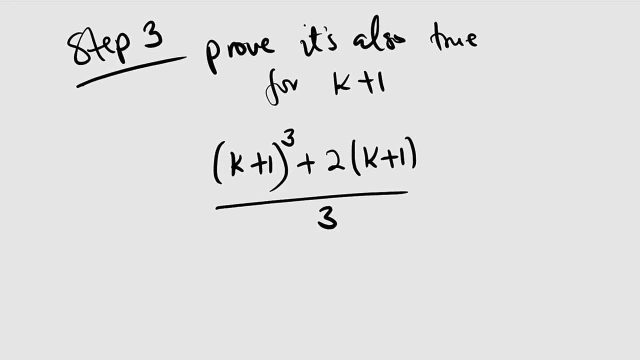 So let's expand this. If you expand k plus 1 to the third power, you're going to obtain k to the third power plus 3k squared plus 3k plus 1.. This is the expansion of k plus 1 to the third power. 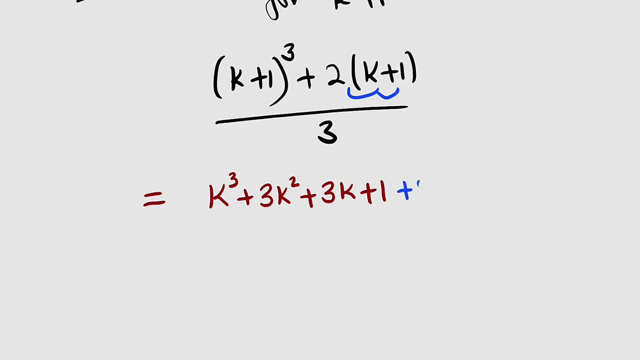 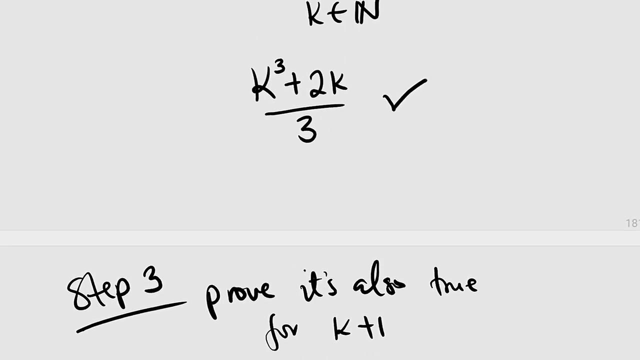 Then if you distribute 2 over this, you're going to obtain 2k plus 1.. We want to show that this is also divisible by 3.. But observe from what we have done earlier. We have seen that k to the third power plus 2k divided by 3. 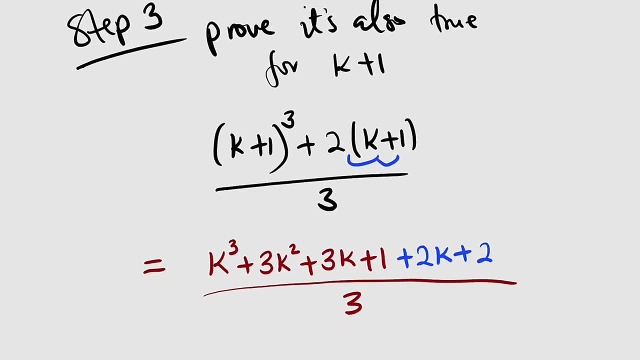 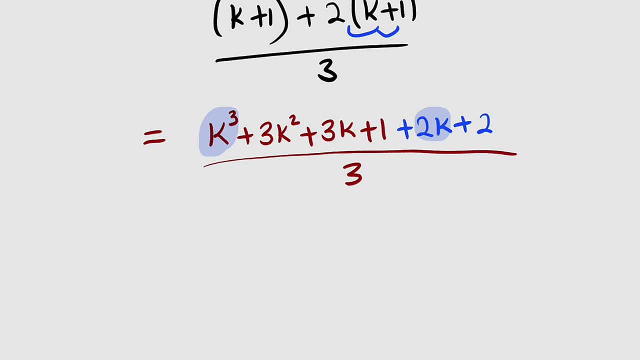 is divisible by 3.. And observe that we have such terms here: k to the third power plus 2k. So we can bring them together. So we have k to the third power plus 2k. Then let's group this together. 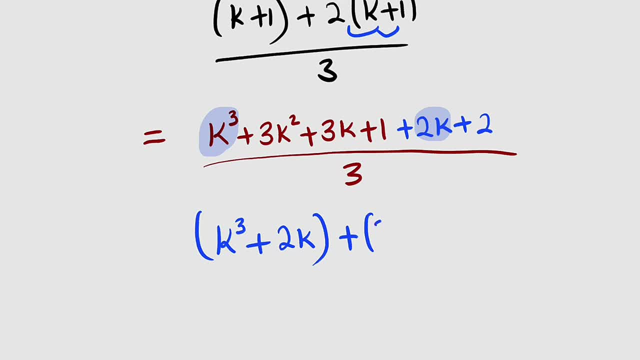 Then plus the other terms, We have 3k. squared from this plus 3k, Then you see we have 1 plus 2, equal to 3. So we have plus 3.. Divide by 3.. We are still proving. 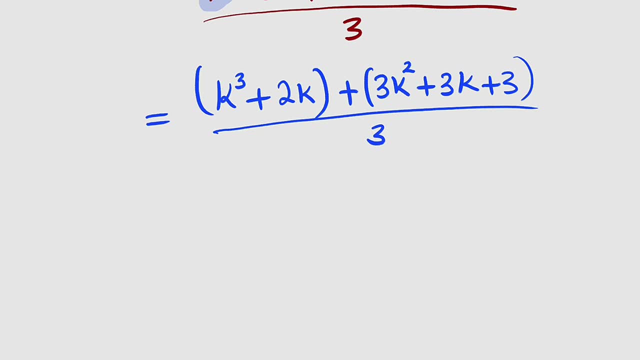 So we can split the fractions Right. So you have k to the third power plus 2k divided by 3.. Right Then, plus the other one, 3k squared plus 3k plus 3, also divided by 3.. 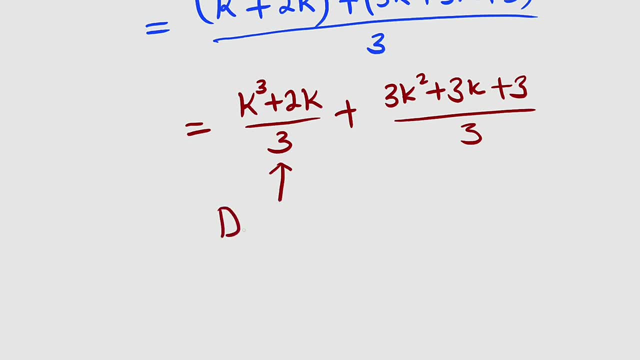 Already. we have seen that this is divisible. We have seen that this is divisible earlier And this can be factorized. We can factorize it as 3 multiplied by k squared plus k plus 3 or plus 1. sorry If you factor out 3 outside. 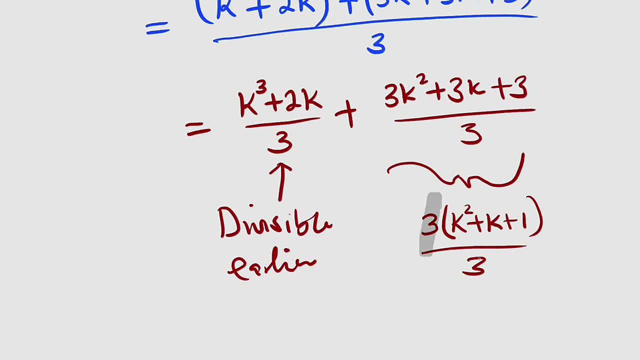 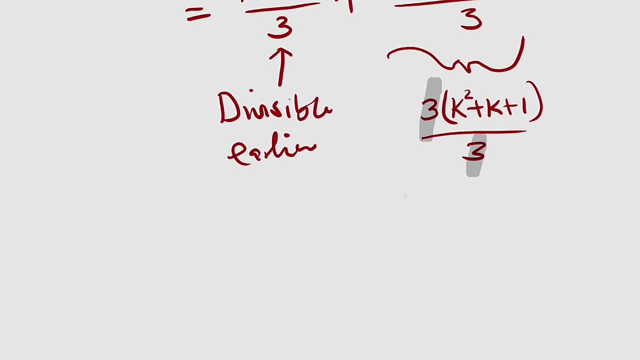 And this is divided by 3. And you can see 3 will cancel 3.. This implies that it is divisible how many times k squared plus k plus 1 times. This is equal to k squared plus k plus 1 times if you divide that by 3.. 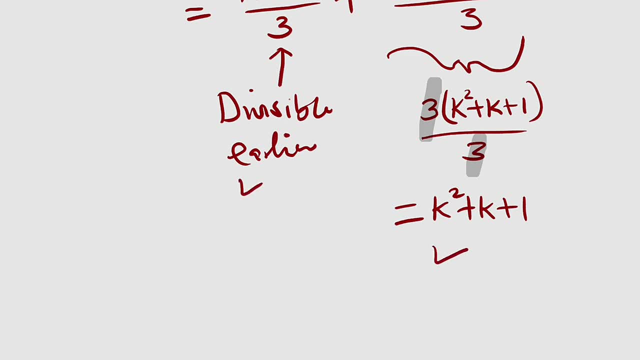 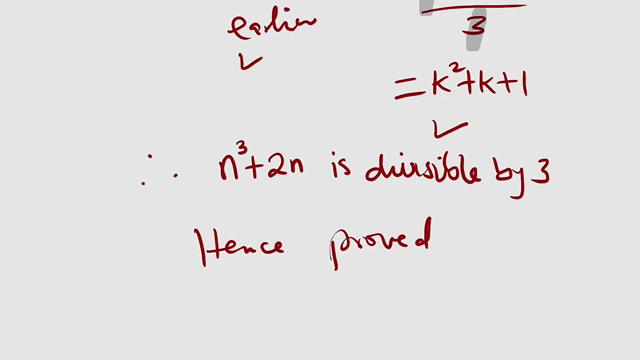 And since this is divisible, this is also divisible. We conclude that, therefore, n to the third power plus 2n is divisible by 3.. Hence proved, And this is all I have for you today. Thank you for watching. Do share to your learning colleagues. 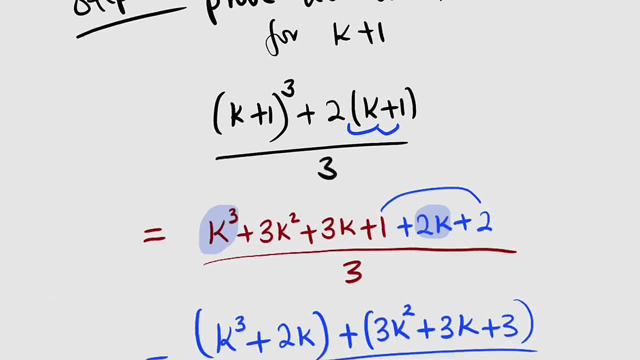 And don't forget to subscribe to my YouTube channel for more exciting videos. Bye, bye.